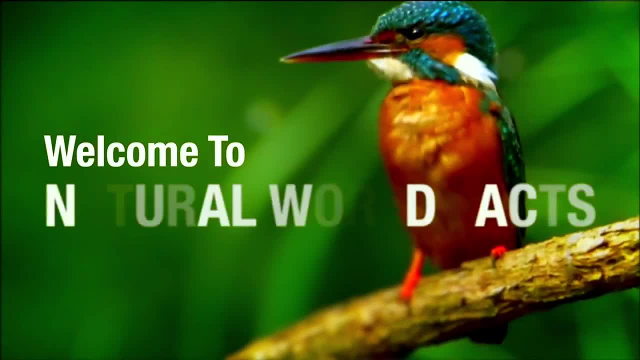 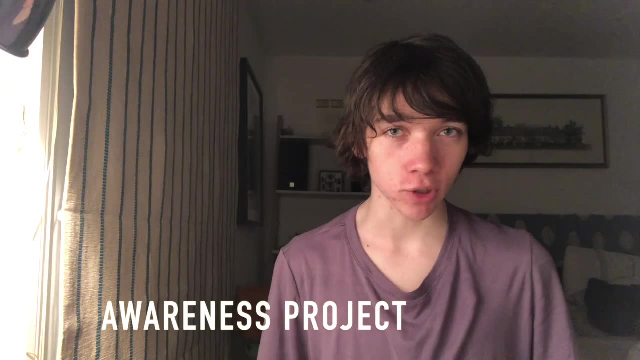 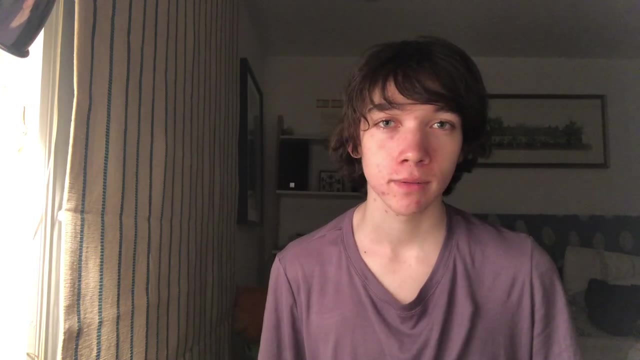 Hello and welcome to the Natural World Facts Awareness Project, a new series in which I'll be explaining the importance of wildlife conservation and what you can do to help. In this video, I'm joined by Alex Collins, a fellow YouTube, wildlife enthusiast and biologist. 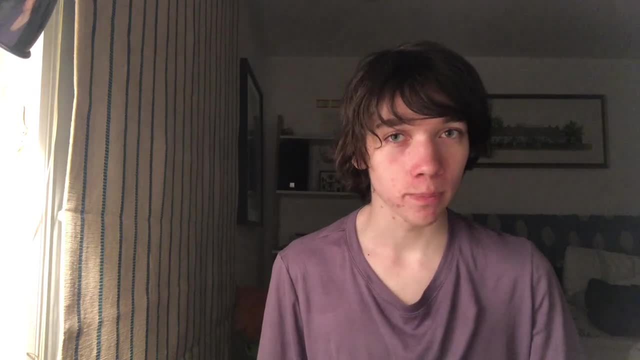 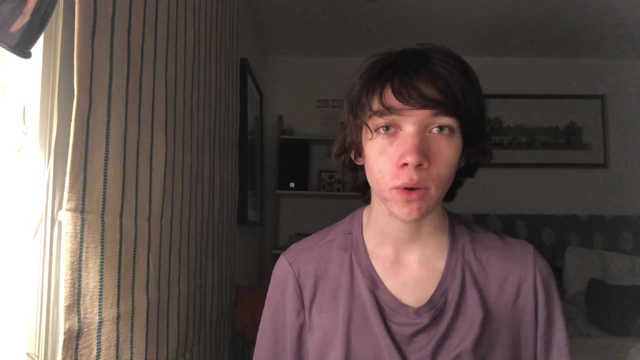 at the University of Bristol. His channel is linked below. I recommend you check it out for videos on some of the world's rarest species and what you can do to help them. So what is marine conservation? Marine conservation is defined as the protection 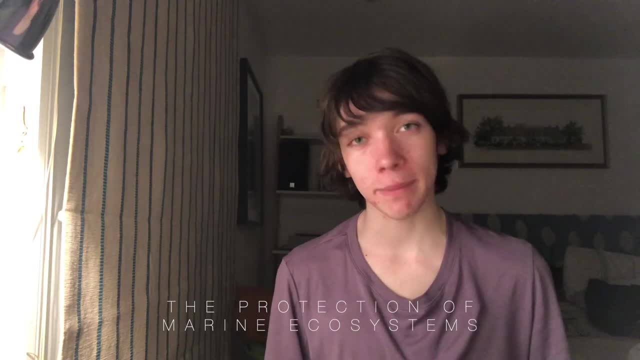 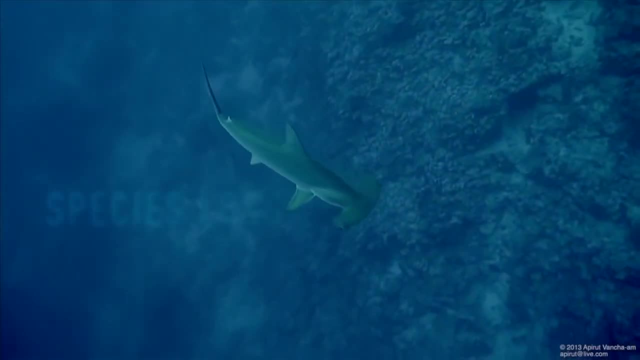 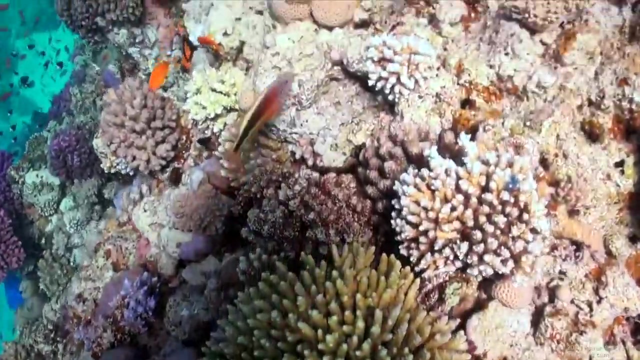 of marine ecosystems, with the focus of limiting the damage caused to them by humans and protecting threatened species. The main threats being seen in our oceans include species loss, habitat degradation and changes in ecosystem function. Human activity is causing a rise in extinction rates. 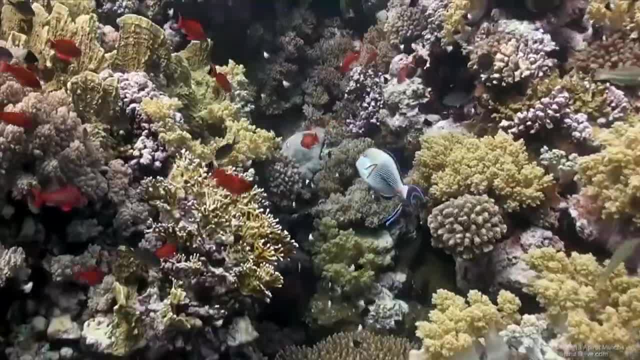 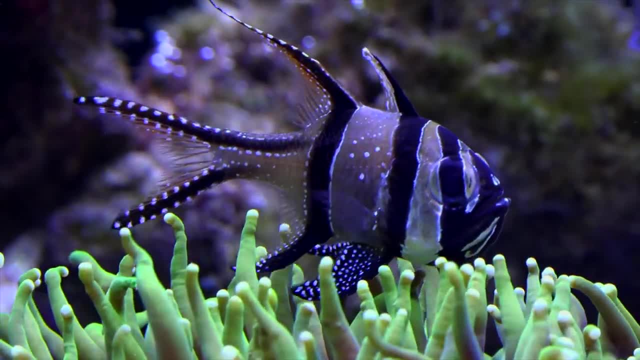 This has led to a huge decrease in biodiversity, particularly in coral reefs, 88% of which are threatened by excessive CO2 emissions. These reefs are among the most important stores of biodiversity on the planet. It takes around 10,000 years for a reef to form from coral. 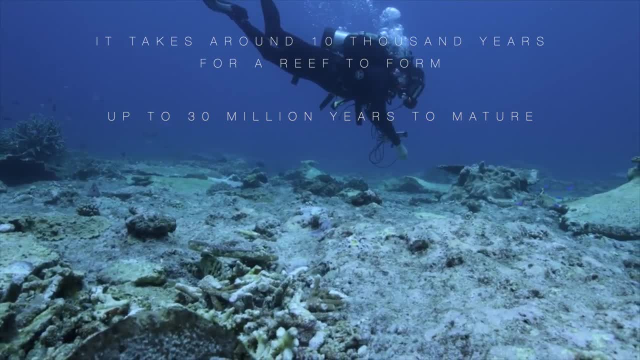 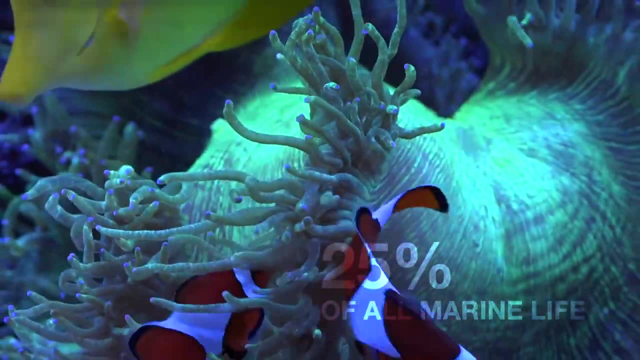 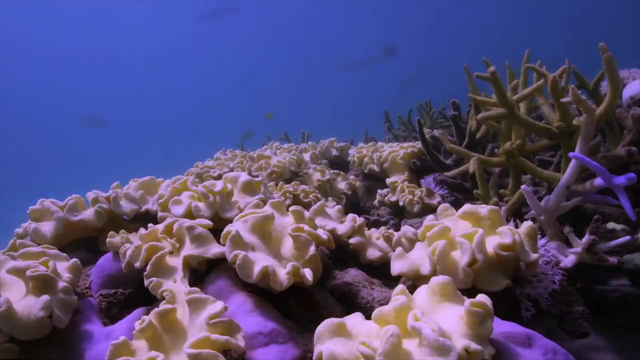 polyps and up to 30 million years for a reef to fully mature, hosting an estimated 25% of all marine life. What is marine conservation? And yet, around the world, coral reefs are dying, as warming temperatures and stressful conditions bleach the corals white as they are forced to expel the colourful algae on. 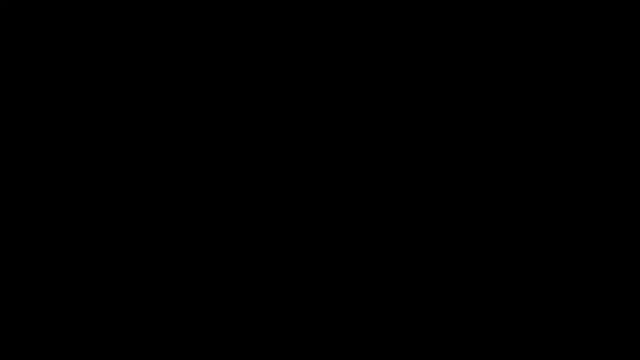 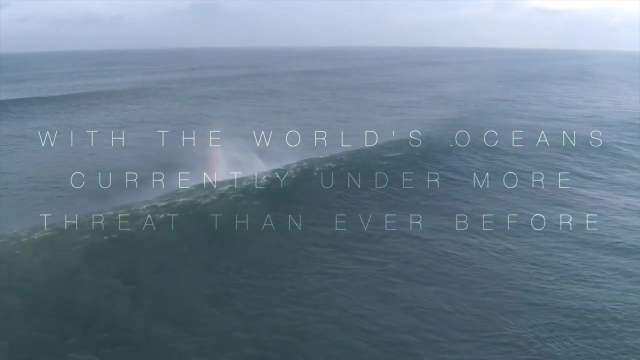 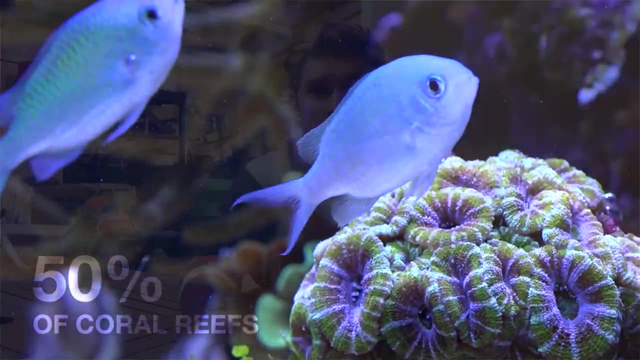 which the corals depend for their survival. So why does this matter? Why is marine conservation so important? With the world's oceans currently under more threat than ever before and with half the world's coral reefs having died in the last 30 years, marine conservation has never been more important than it is today. 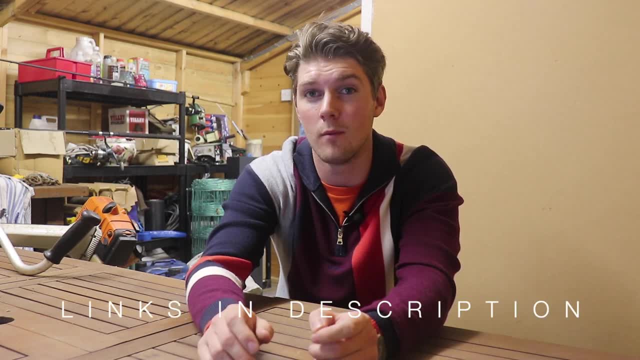 I've already mentioned that marine conservation is a very important part of our lives, and I've already made some videos explaining why conservation is so important to you and why we should save endangered species, so make sure to check out those videos after watching this. 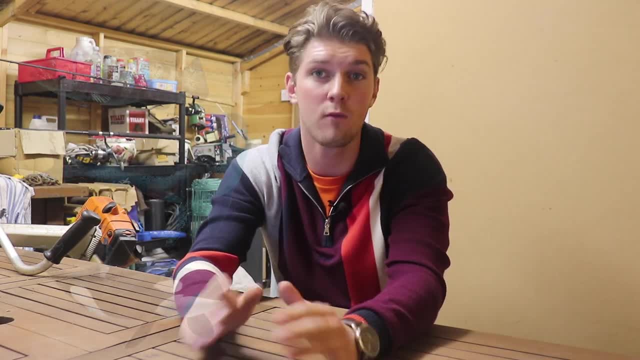 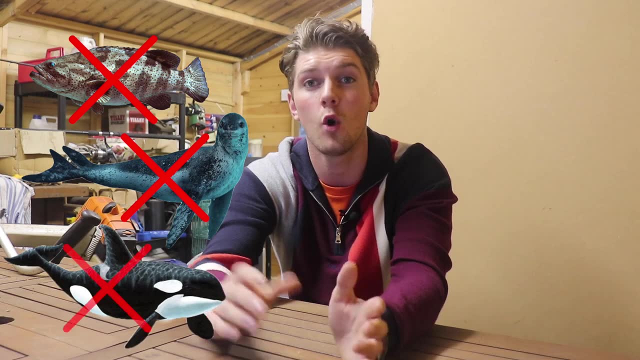 Put simply, different species rely on each other for survival. If one species is under threat, the likelihood is that so is another species. This can have a chain reaction until, eventually, a whole ecosystem is under threat. We need healthy ecosystems just as much as 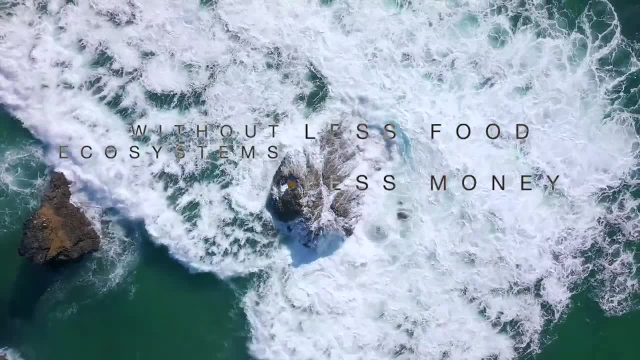 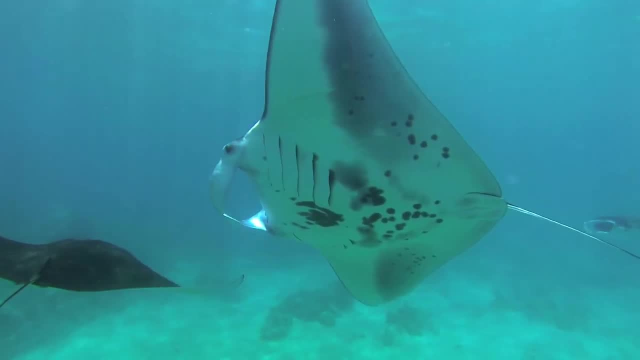 the marine life itself, because without them, we'd have less food, less money and altogether less life on our planet. The bottom line is: earth needs healthy oceans, and it's our responsibility to protect them. So how can we do this? One of the most effective methods has been the setting up of marine 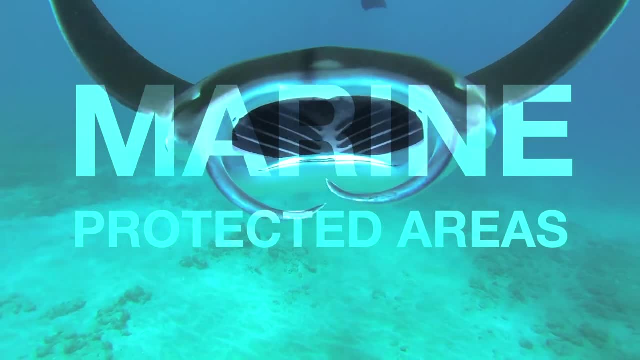 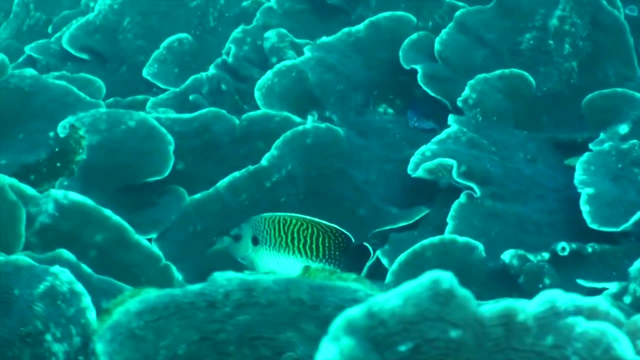 protected areas. This creates a much safer environment for marine life, undisturbed by the impacts of overfishing, noise, pollution from ships and other human activities. Thankfully, biodiversity has been found to increase by 21% within marine reserves like these. We. 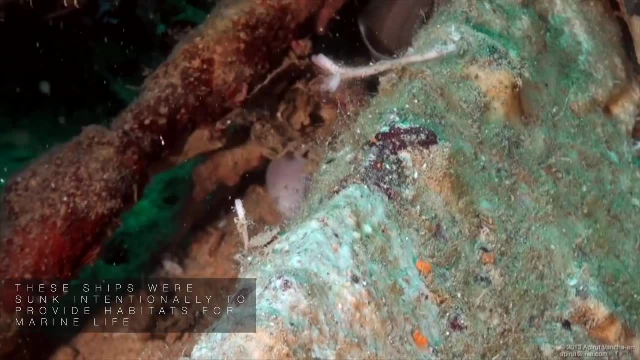 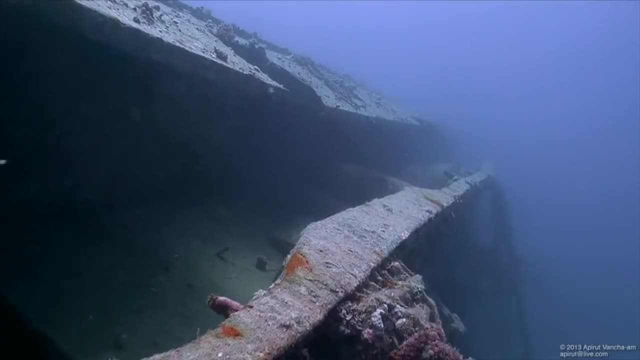 can also use artificial reefs. That means that the marine environment can be used to protect the ocean from all kinds of. These are man-made structures built to promote marine life and the growth of new coral. Artificial reefs have proven successful in providing a habitat for threatened wildlife. 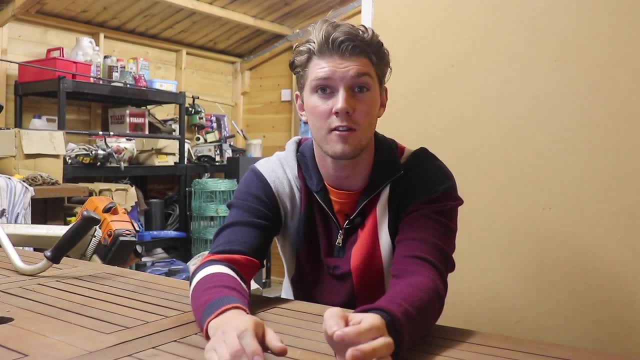 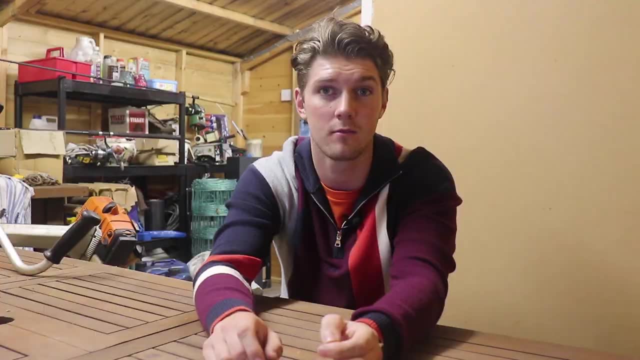 This allows damaged ecosystems to recover and valuable biodiversity to regenerate. As well as these strategies, we also need to be careful in the way that we interact with our marine environment. Active demersal fishing techniques like trawling, where a net is dragged along the bottom of the sea floor. can be really destructive, as this destroys ecologically important species like certain corals. Active pelagic fishing techniques where a net is dragged through the open ocean can also be just as bad. This is because they're indiscriminate, meaning they'll catch anything in the way of the net. 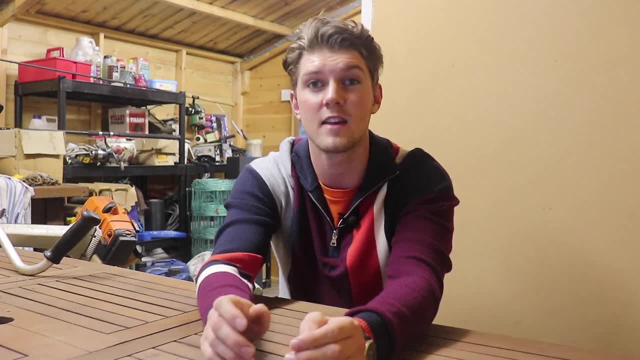 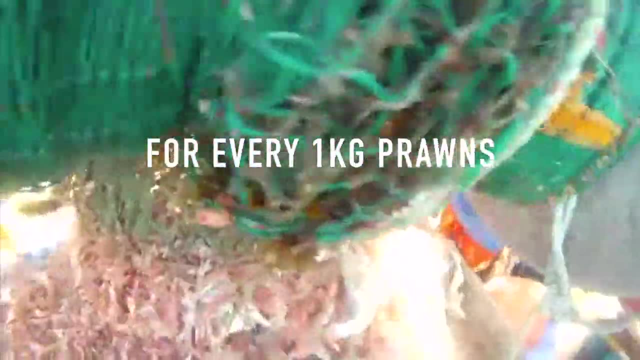 regardless of whether the fishermen want it or not. This often leads to protected animals like dolphins and turtles being injured or killed. For every 1kg of prawns that are caught and sold in stores, 9kg of other sea animals are caught. 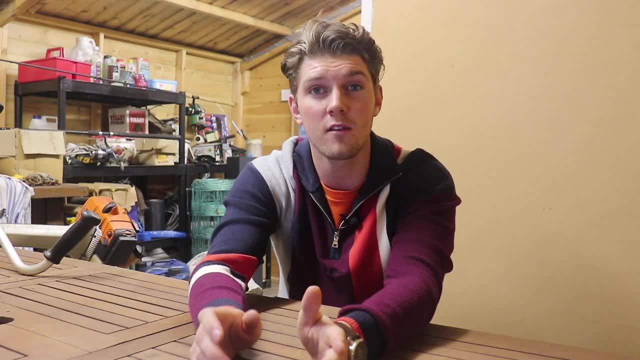 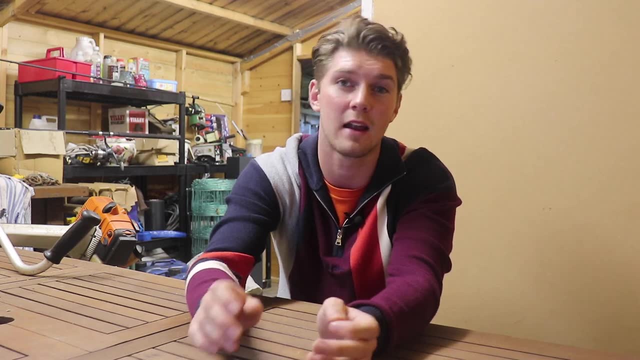 This is considered as by-catch- being injured or killed and then thrown away. Marine conservation efforts have been made to reduce the destruction caused by these fishing techniques, either by reducing the amount of times that these techniques are allowed to be used or making the techniques themselves less destructive. 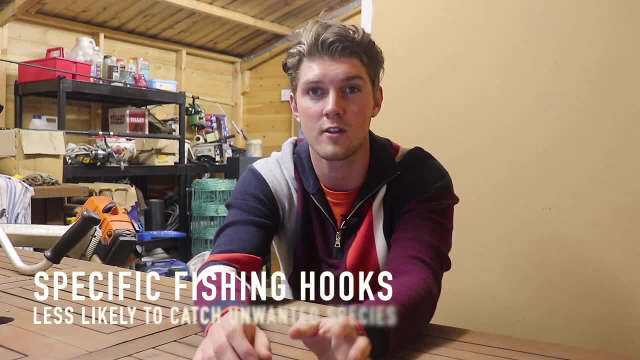 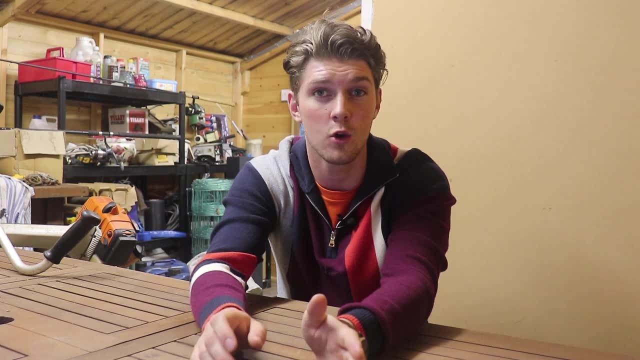 One example of this is the use of specific fishing hooks, which are less likely to catch unwanted species. Solving these problems does take a lot of hard work, but that doesn't mean that there's nothing that you can do if you don't work as a conservationist. 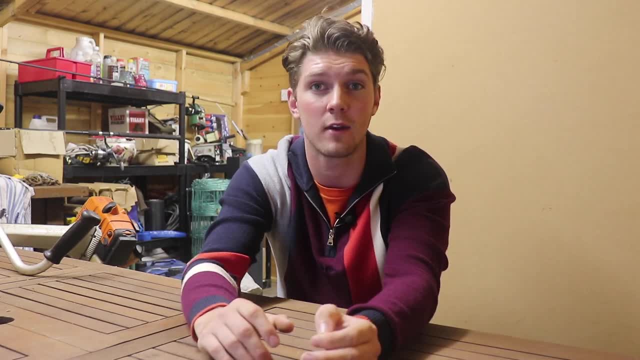 So here are some of the things that you can do to reduce the amount of time that these fishing techniques are allowed to be used. So here are some of the things that you can do to reduce the amount of time that these fishing techniques are allowed to be used. 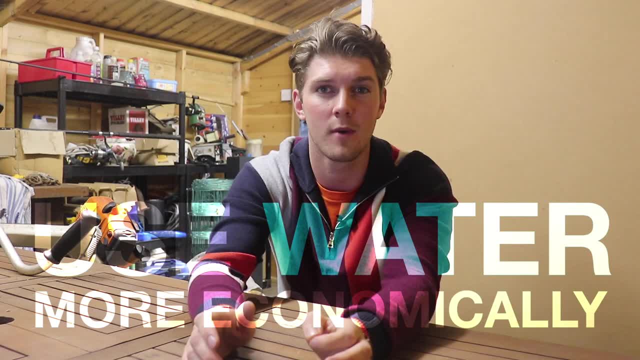 So here are some of the things that you can do to reduce the amount of time that these fishing techniques are allowed to be used. Firstly, use your water supply more economically. This will not only save you money, but it will also reduce excess runoff containing pollutants and waste into the ocean.